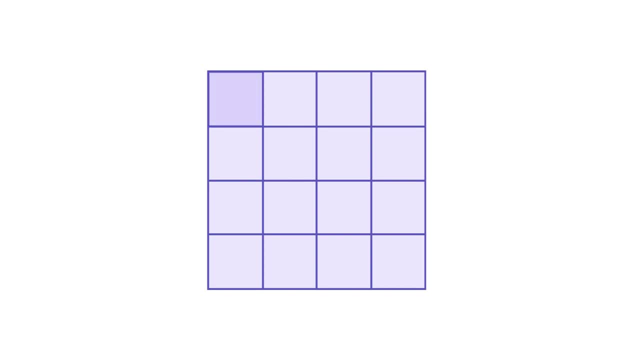 A CCD is made up of a large grid of individual light-sensing elements called pixels. When light hits a pixel, the photon of light is converted into an electron. Each pixel on a CCD will have had a number of photons in it. These photons fall on it during an exposure. 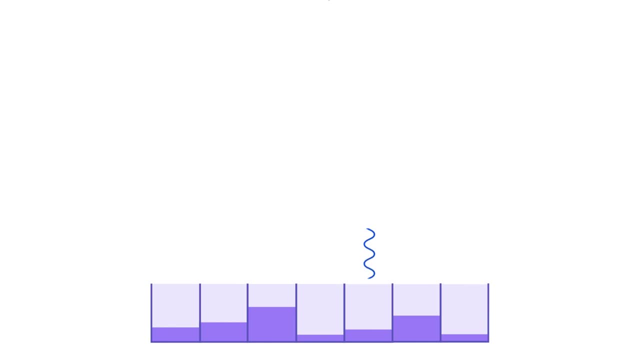 This number of photons translates to a number of electrons that are stored in the CCD until it is read out. The more photons hitting a certain pixel, the more electrons are stored there. To measure the amount of light that fell onto each pixel, the number of electrons is counted. 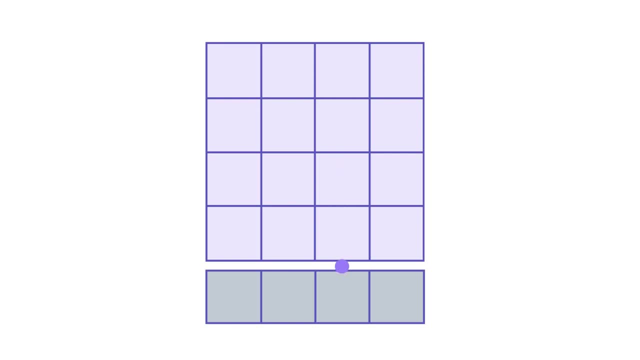 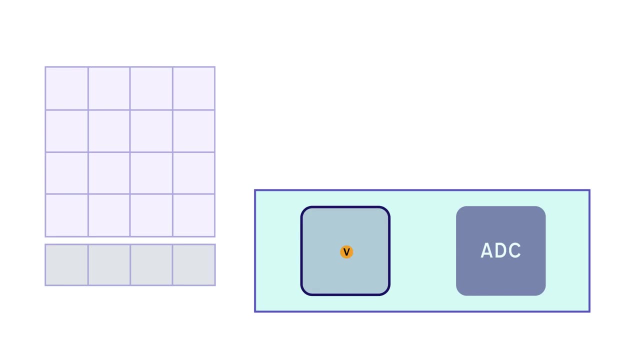 The electrons are moved down the column of pixels to a read-out register. They are then moved one by one to an output node, where they are converted to a voltage through a capacitor, and this signal is passed through an amplifier to make it larger and easier to measure. 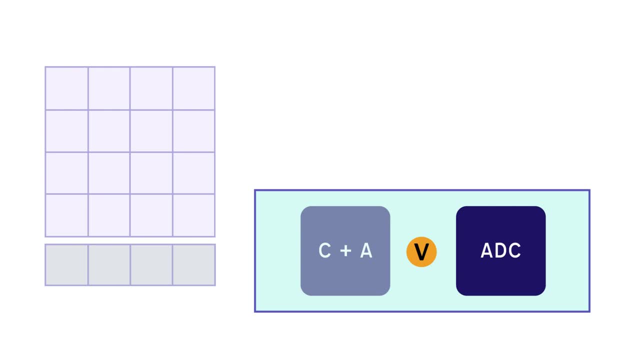 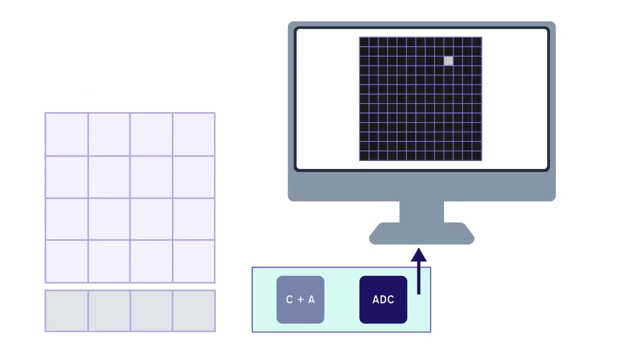 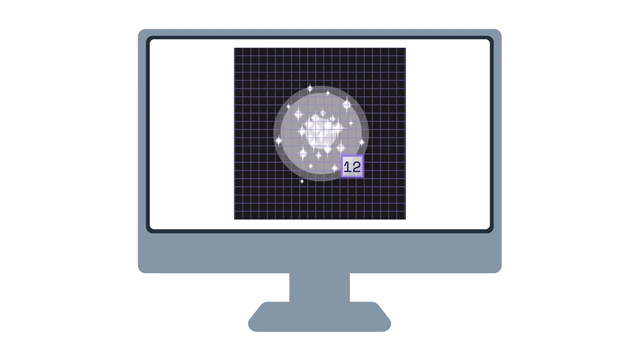 An analog-to-digital converter converts this voltage to a number. We can convert this number into a colour or a brightness to show it on a computer screen. A darker pixel in the image indicates a low number of photons and a brighter pixel indicates a higher number of photons fell on the pixel. 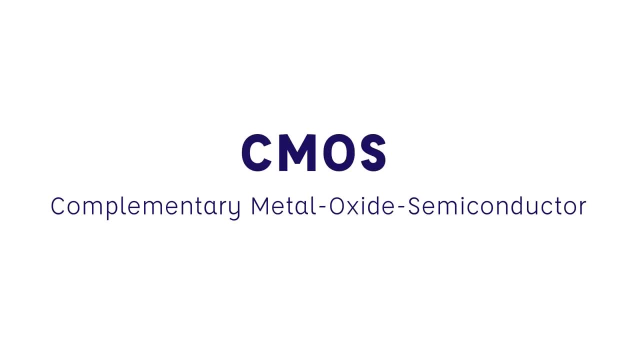 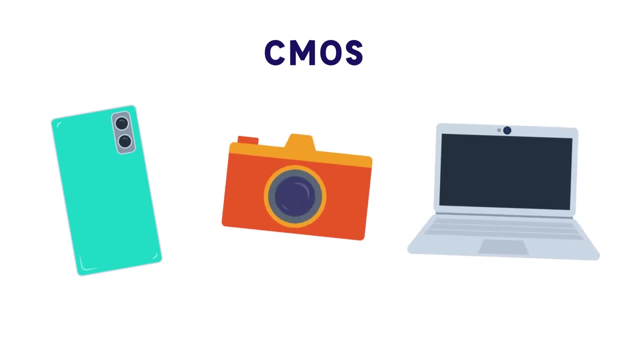 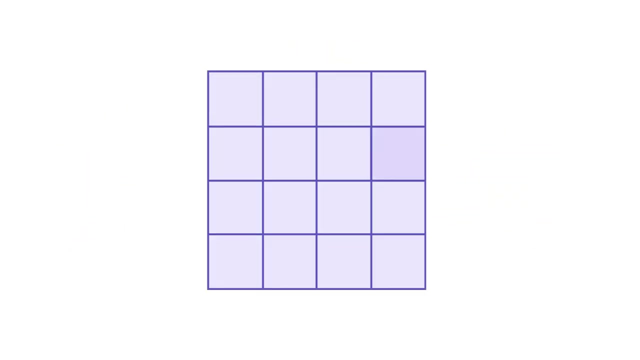 A CMOS device is another type of camera sensor used in astronomy. CMOS devices are also used in digital cameras such as mobile phone cameras, webcams and digital single-lens reflex cameras. Similar to a CCD, a CMOS sensor uses a grid of pixels. 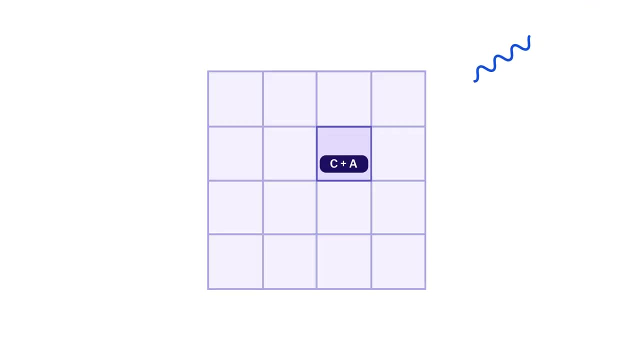 But unlike a CCD, each pixel contains its own capacitor and amplifier. This means that when photons hit the pixels, they are converted to electrons and then immediately into a voltage at each individual pixel. Every column of pixels also has its own analog-to-digital converter. 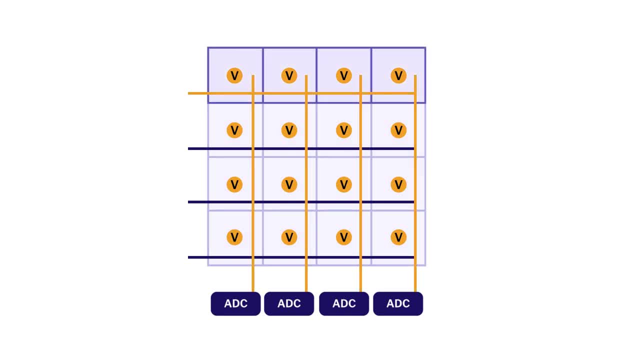 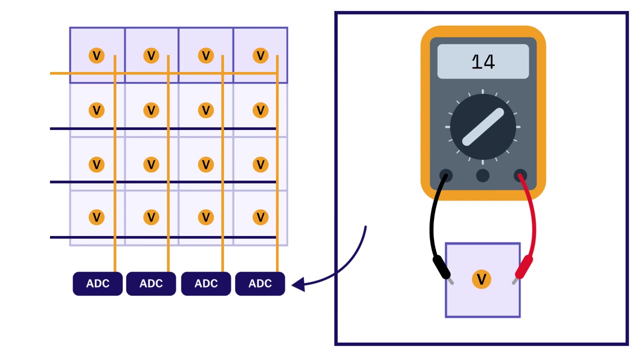 These switches direct the voltage to the ADC row by row, where they are converted to a brightness value by each ADC. You can imagine this like having a digital multimeter or voltmeter connected to each pixel in the row showing the analog voltage signal as a number on screen.